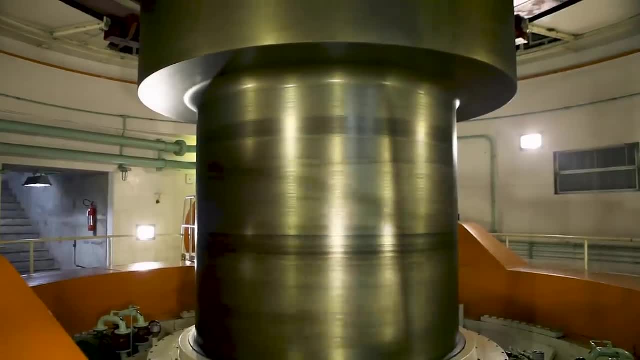 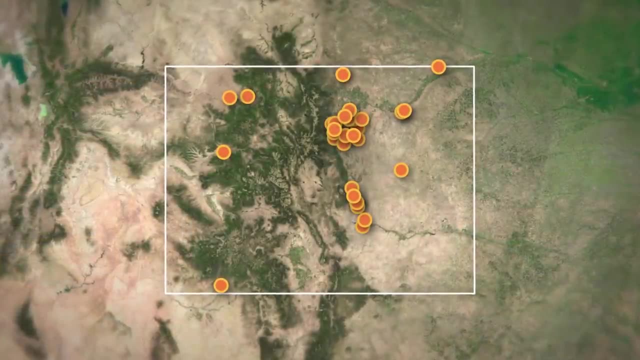 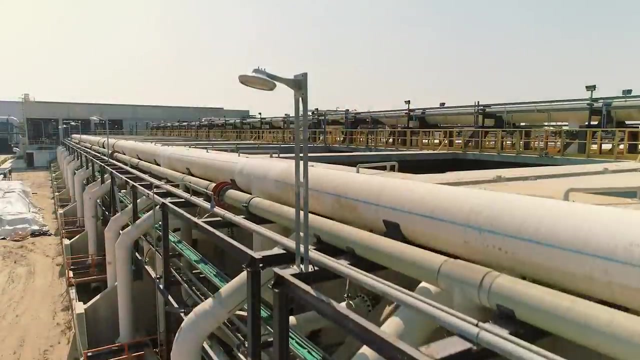 If you flip a light switch in Los Angeles, that could cause a turbine in Washington to start spinning. Electric grids are considered some of the single largest machines in existence—they stretch across entire continents- but they're machines with absolutely zero slack With water systems. for example, there's some extra supply in a storage reservoir at the treatment plant. 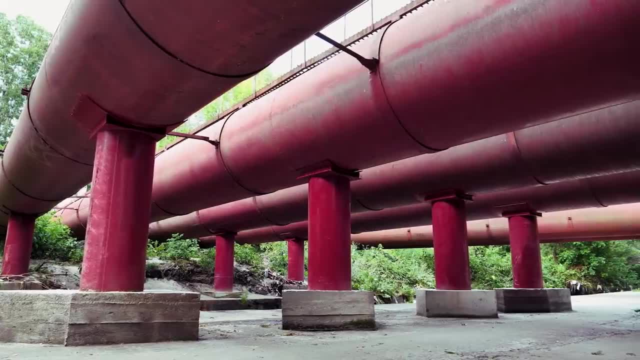 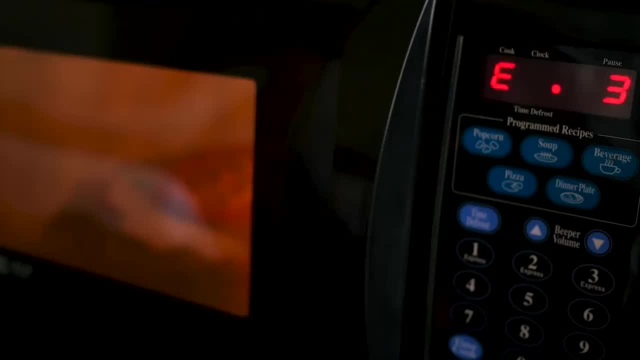 and some extra supply in the pipes connecting the treatment plant to your home—supply only has to roughly match demand—but that's not the case with electricity. Your lights, your TV, your microwave—everything plugged into the grid uses electricity produced just moments ago. For the sake of example, let's look at what it takes to turn a light switch in Los Angeles into a power grid. For the sake of example, let's look at what it takes to turn a light switch in Los Angeles into a power grid. For the sake of example, let's look at what it takes to turn 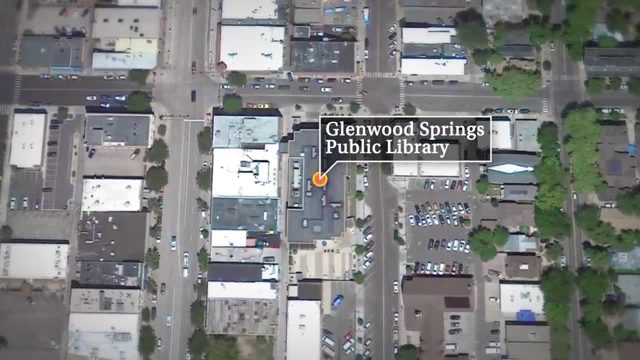 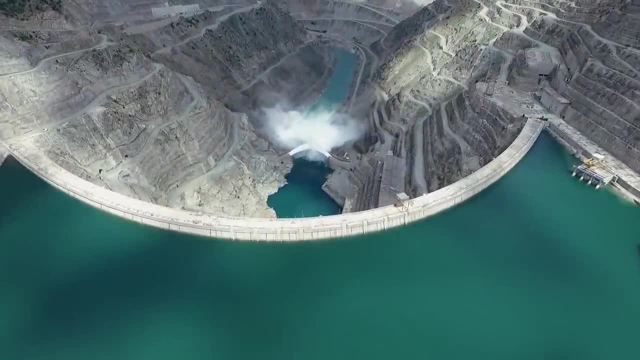 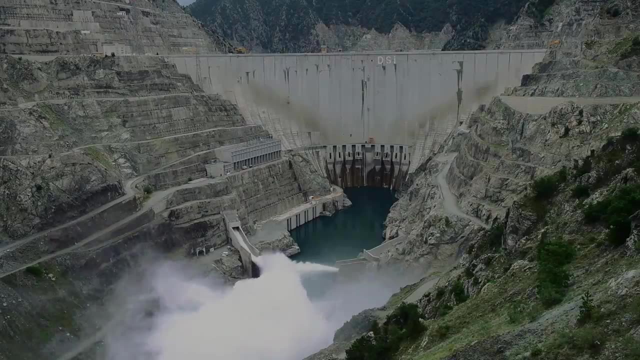 the lights at the public library in the small town of Glenwood Springs, Colorado. Now, what makes the relatively straightforward task of converting natural fuels or phenomena into electric power difficult is the huge variability in demand from minute to minute and month to month. There are, however, some trends On an annual basis. 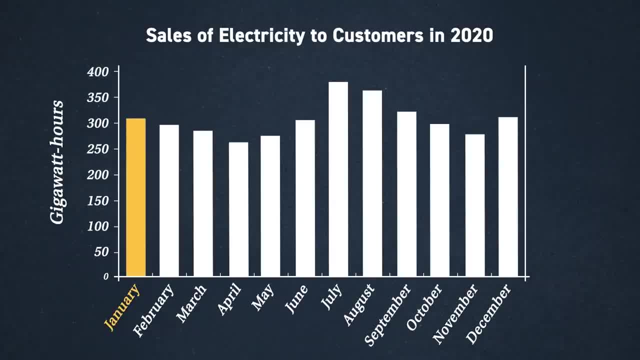 the peaks correlate to climate—January represents the winter high water mark, as many homes and businesses turn on their electric heating, while July typically ranks highest out right as the country battles summer heat with air conditioners. The month-to-month variations are not that significant though—the difference between 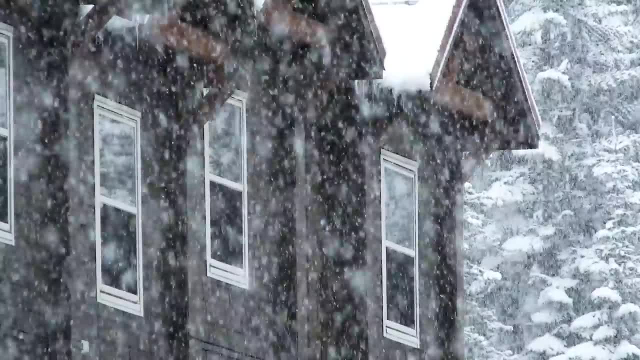 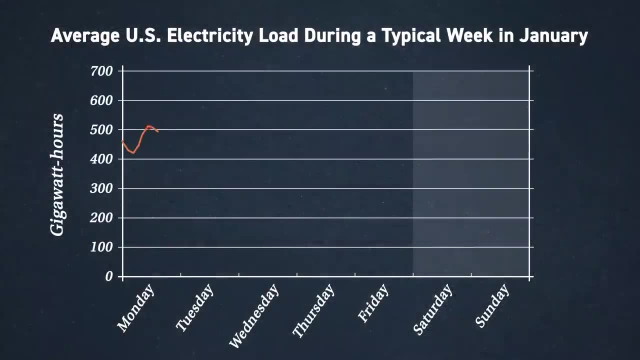 the highest and lowest demand months is less than a third. Most of the variability happens across a given day. In January, all regions of the US observe a two-peak daily demand trend where electricity use spikes around 7am as people turn off their thermostats and fire up lights and appliances. 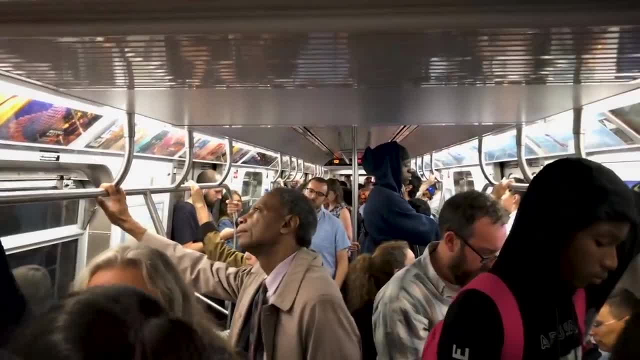 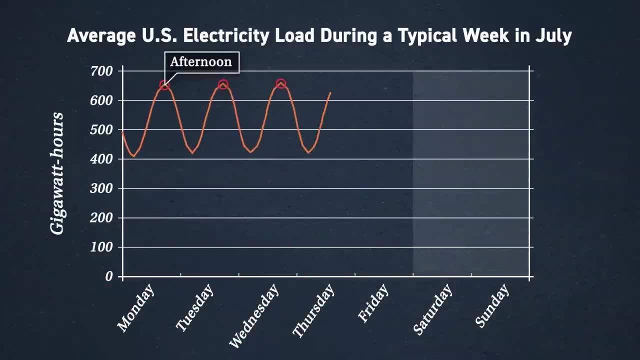 as they wake up and get ready for the day. Then demand peaks again when people return from work in the evening and do the same Meanwhile. in July, energy use is highest in the late afternoon or early evening, but this does depend on the region. 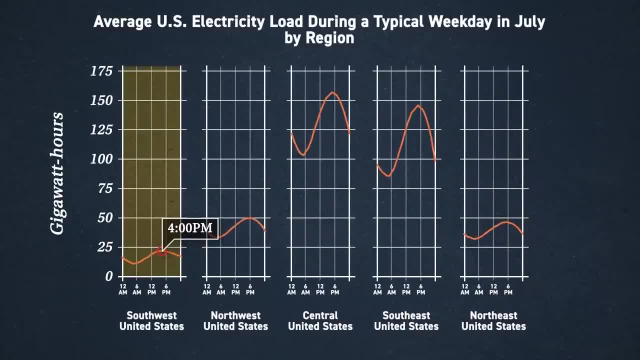 For example, in the sweltering southwest, usage peaks around 4pm—around the hottest hour of the afternoon- when air conditioners have to work the hardest. In the more temperate northwest, though, which includes Colorado and that Glenwood Springs- 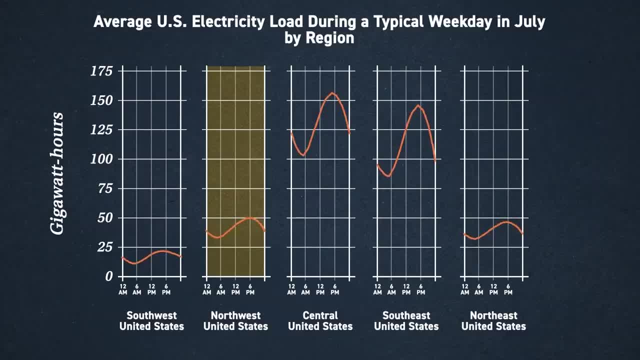 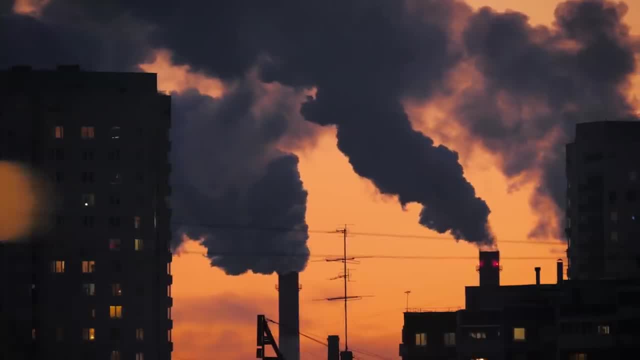 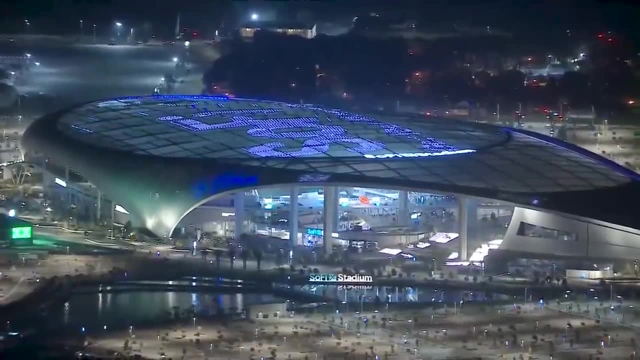 public library. fewer buildings have air conditioning, so demand peaks around 6pm—pulled back by post-work evenings. These trends then get further complicated by holidays and special events. For example, on Super Bowl Sunday in the US, demand plummets for a few hours as people 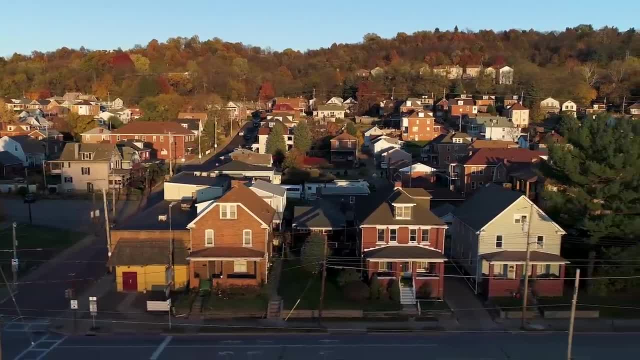 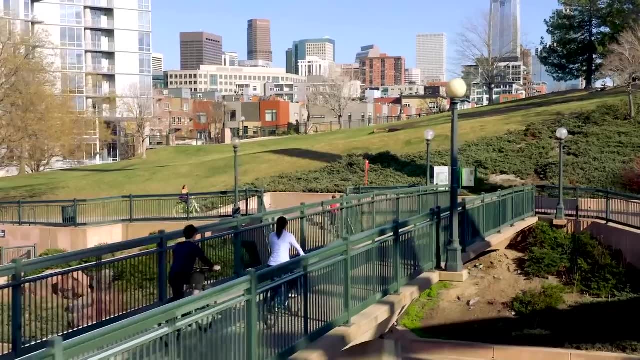 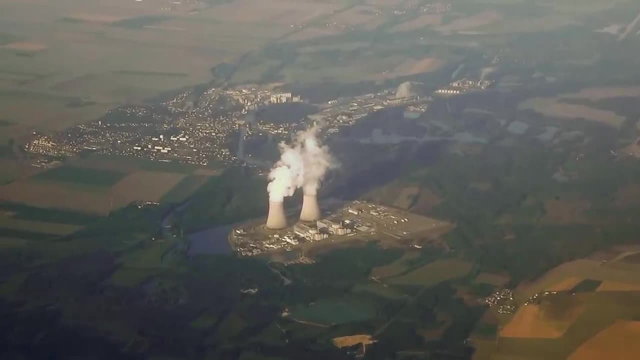 turn off the lights, stop cooking and gather together at others' homes to watch the big game. This is all to say. when forecasting demand, utilities need to factor in the hour day, season, location and plenty more. Now, with whatever demand materializes, utilities then need to essentially instantly calculate. 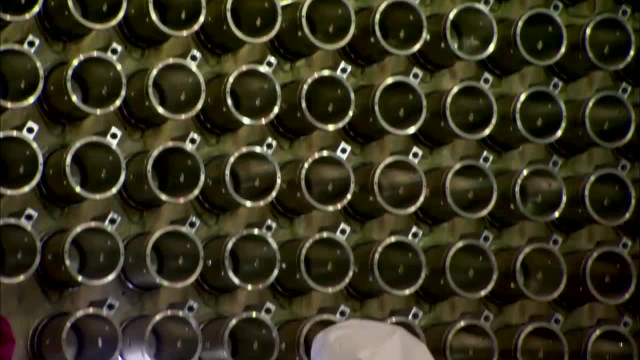 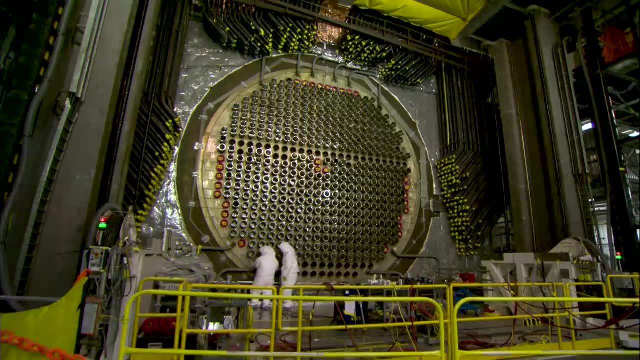 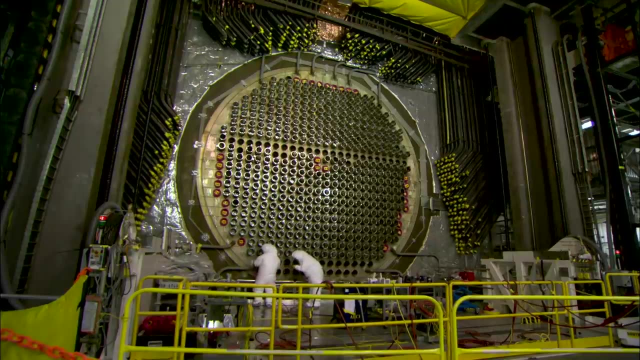 how much energy they need to supply. To do this, they layer different energy sources on top of each other. Often, the lowest layer is nuclear power. Nuclear power stations aren't designed to be able to turn off and on easily—it would take the better part of a day to shut down and start up again, so it's rather impractical. to operate these in response to demand. In addition, considering how massively expensive their construction is, it would be economically inefficient to let these stations run idle. Therefore, they'll run nearly continuously for the entirety of their service lives, except for during planned maintenance. 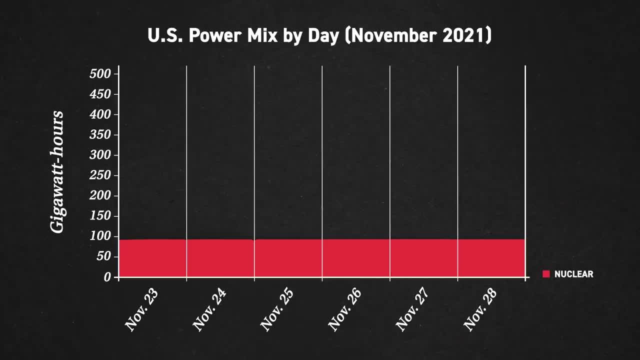 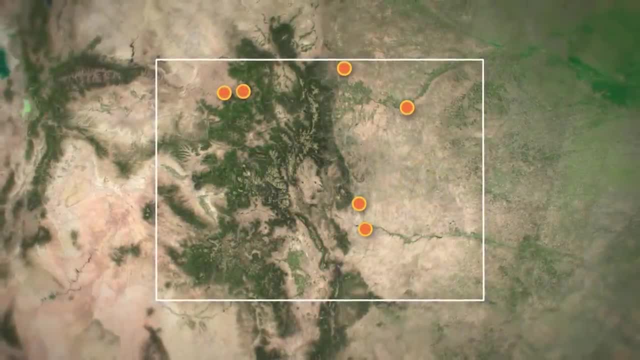 This means they provide the most stable supply of electricity, 24-7.. Colorado no longer operates any nuclear power plants, but it does have six of the next layer—coal power stations. Like nuclear, most of these coal plants cannot be fired up quickly, as they take some time. 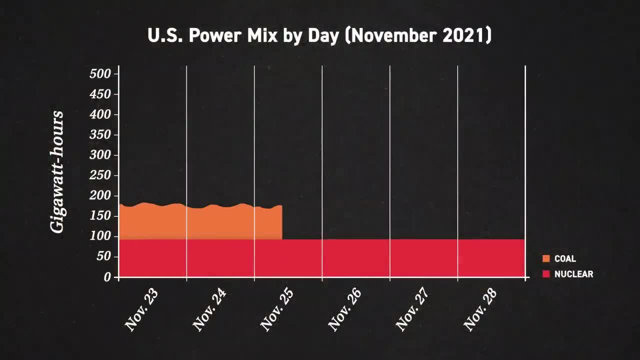 to get up to temperature. so utilities will also run them essentially continuously. Coal and nuclear combined They'll basically fulfill what's called the baseload. Their continuous production essentially equals the valley of demand—they'll make the minimum amount of power needed at a point in the day. So then, on top of that, utilities need production methods that can fire up and shut down far faster. They need to be able to produce the power to operate all those AC units in hot summer afternoons. The bulk of this job is completed by natural gas-fired plants. 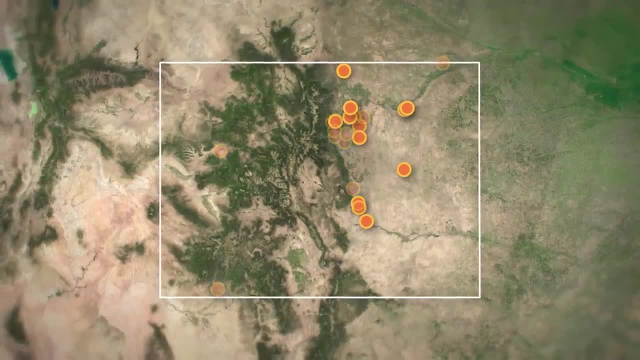 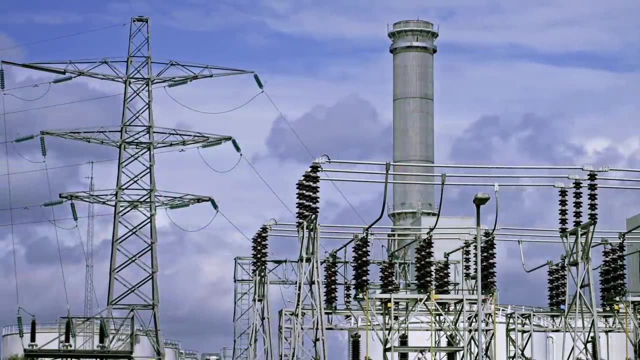 Of the 25 in Colorado, 13 of these stations are coal-fired. The bulk of this job is completed by natural gas-fired plants. 15 of these stations generate using a simple-cycle combustion turbine. This is the simplest means of turning natural gas into electricity. Much like a jet engine. the fuel is used to turn a turbine which turns a generator which produces electricity. More advanced natural gas power plants recover the hot exhaust to convert it into electricity too, but the startup process for these takes longer, so simple-cycle stations are used. 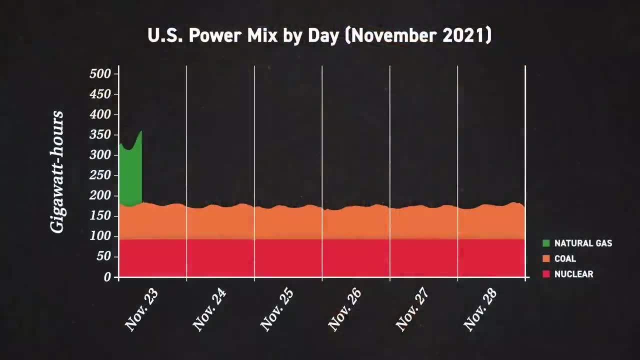 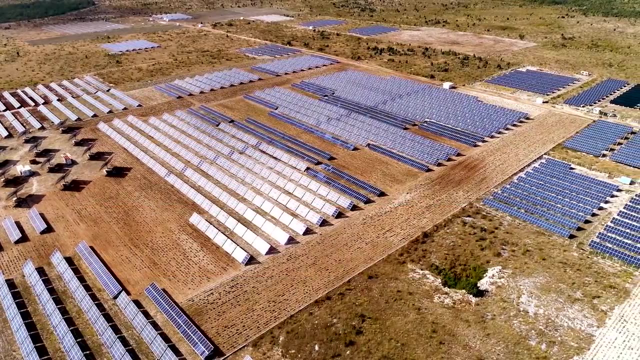 for applications where speed is key. Most can reach full power within 15 minutes, making them an effective way to generate more power. Nuclear, coal and natural gas are some of the more traditional means of generating electricity. The recent proliferation of renewable energy sources, though, has kickstarted a reinvention. 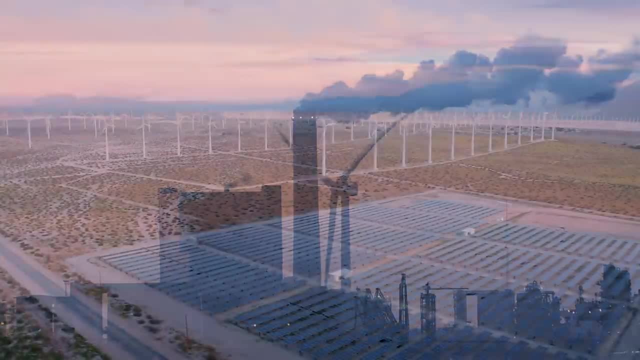 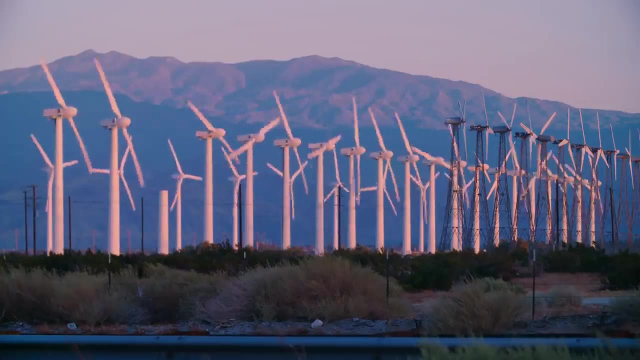 of this system of baseload and peaker plants. That's because, when wind and solar generating stations can make power, that power is essentially free—meaning there's essentially no additional variable cost to generate power once the panels or turbines are installed. 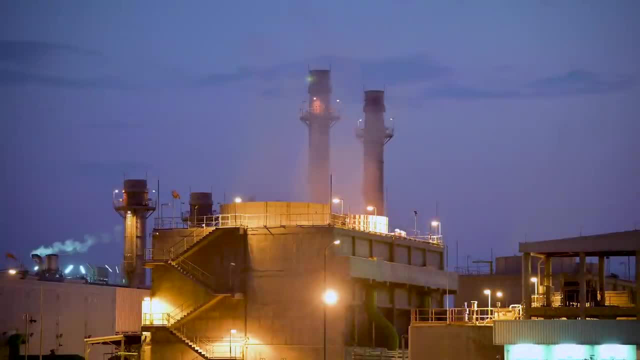 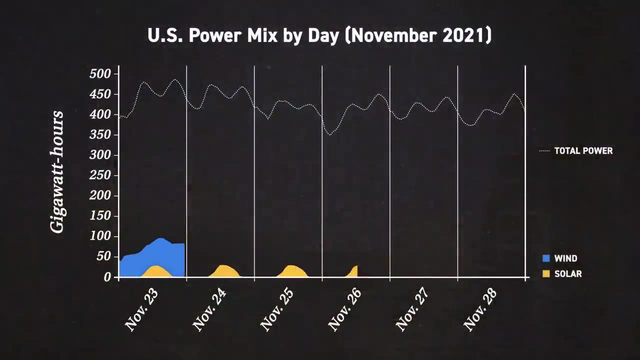 That's not the case with natural gas-fired plants, for example, as the gas itself represents one of their primary costs. So this essentially creates a new bottom layer to the energy mix, but it's a bottom layer that's uncontrollably variable. 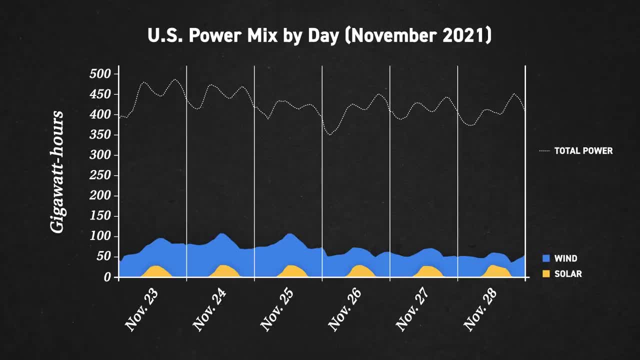 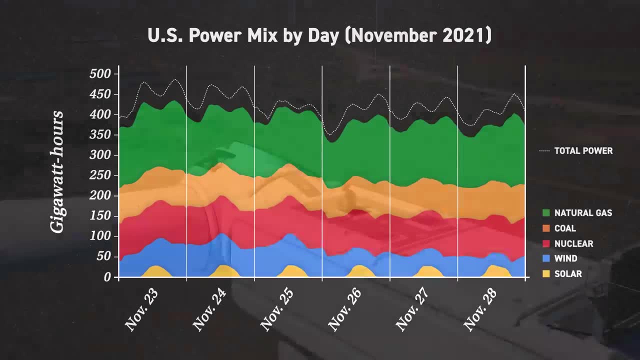 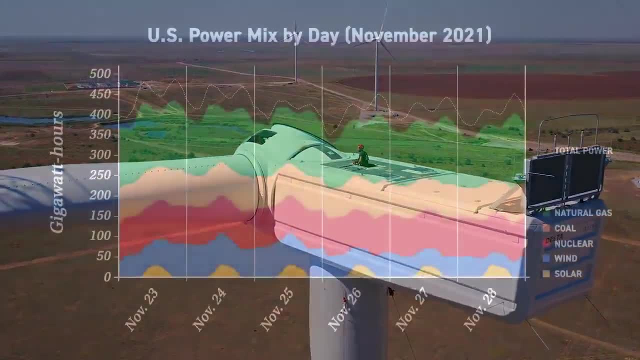 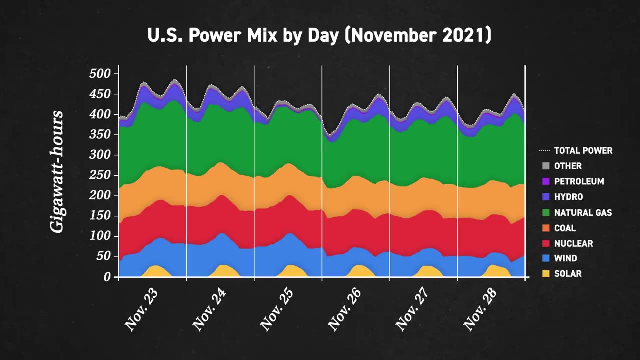 The natural gas and electricity are the cheapest sources of electricity but because they rely on natural phenomena, they can't match supply to demand the way that the traditional nuclear coal natural gas trifecta can. Therefore, grids are being reinvented so that supply doesn't have to match demand—at. least minute to minute. Of course, the way to do that is with storage, but storing electricity is not easy. The average American household uses about 30 kilowatt hours of electricity per day. System ion batteries currently cost around $130 per kilowatt hour, meaning one day's. 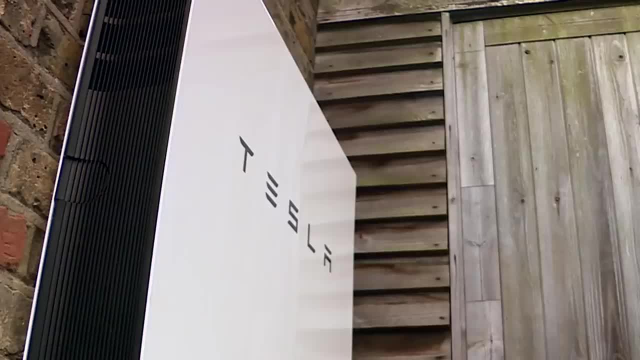 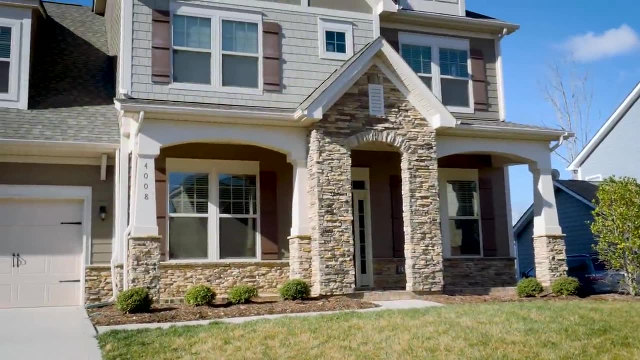 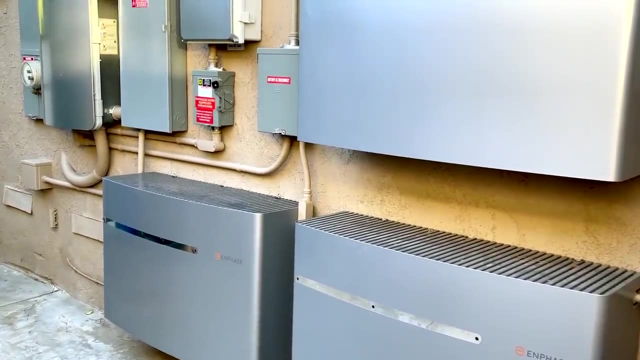 storage for one household would cost around $3,900 in batteries—and that's excluding all the additional infrastructure needed to make such an installation possible. Considering the average American household pays less than half of that per year in electricity bills, installing such a system grid-wide would be economically impractical. 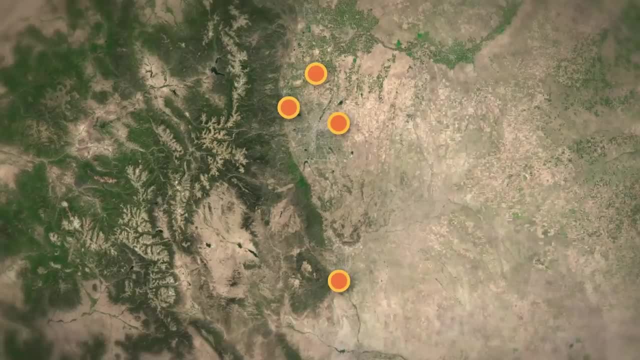 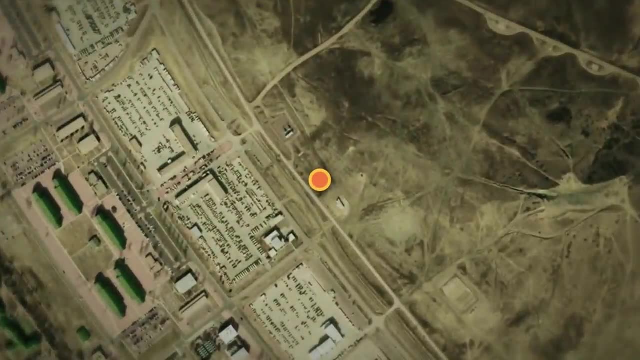 Nonetheless, Colorado has four battery electric storage systems, albeit at a relatively minor scale, The largest of which is used to power Fort Carson, a US Army base near Colorado Springs. They charge up the 8.5 megawatt battery at night when electricity demand, and therefore 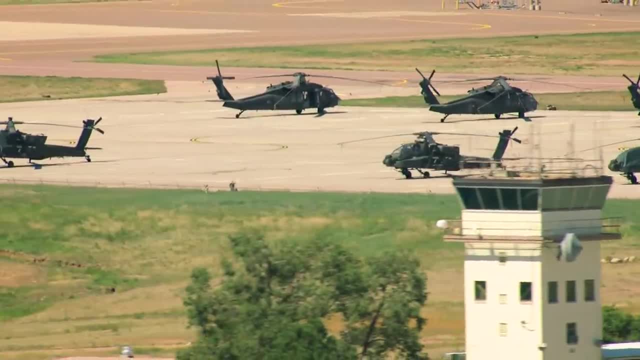 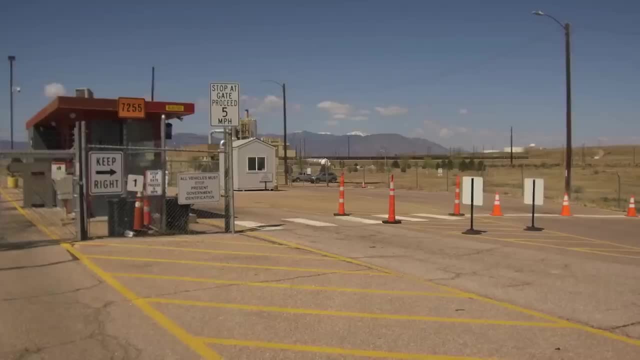 rates are low, then use the power during the day when the majority of the base's electricity use occurs. The system's savings should make up for its installation costs in about 13 years, and by the end of its practical lifespan it's expected to have saved the Army about. 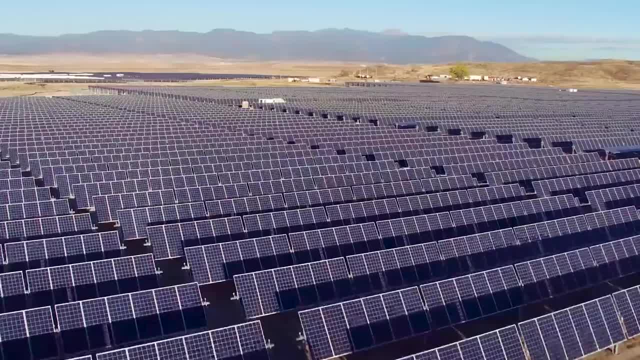 half a million dollars in electricity costs. While such a system can make economic sense for large companies, it's not the only way it can make a difference in the lives of the people it's going to be able to save. It's not just the fact that it's a system that can build power complexes, that can invest. 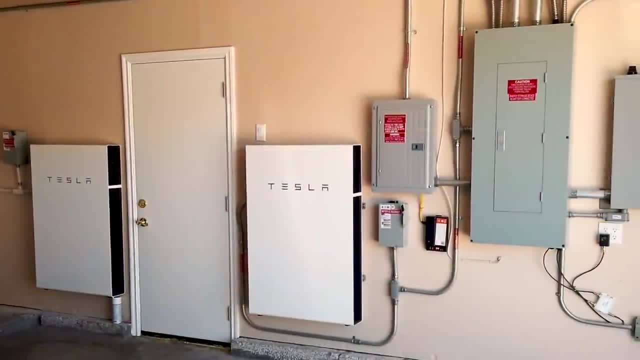 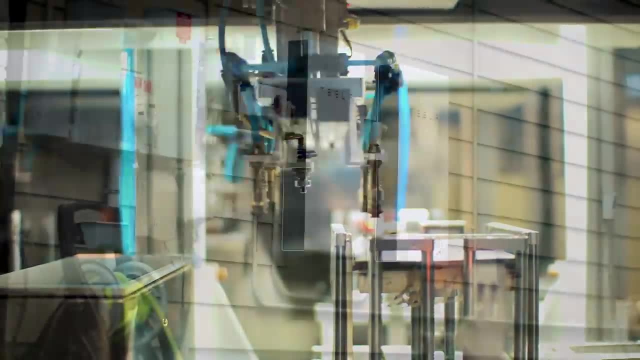 in infrastructure that won't pay off for more than a decade. it's just not practical grid-wide—at least right now. Even if there was the battery production capacity to make a meaningful dent in the world's electricity use, the savings just happen too far in the future for most to consider such. 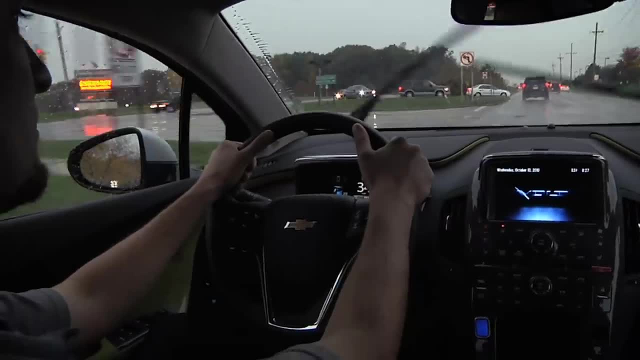 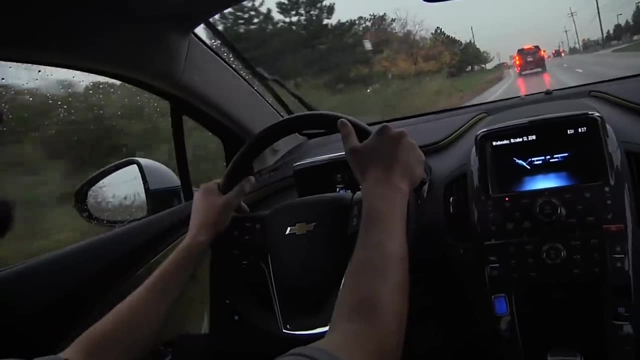 storage to be worth it. However, for entirely different reasons, in the coming decades, more and more people will be purchasing massive battery packs—the ones inside their EVs- with most forecasts suggesting that some third of the battery would be used for electric vehicles. 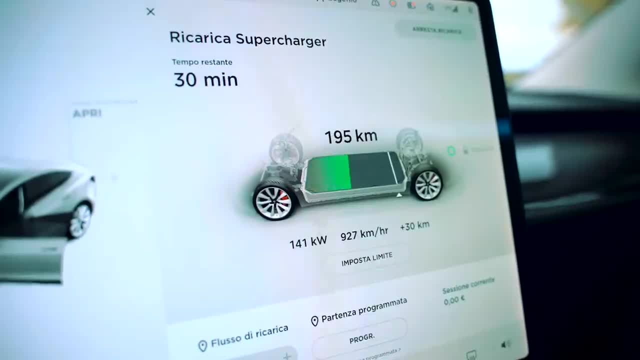 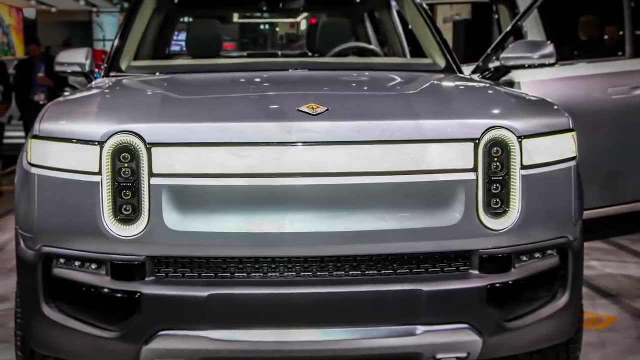 While a third of new car sales in the US will be electric by 2030, a potential solution to the grid's storage need could arise naturally. A Rivian R1T, for example, holds a 135-kilowatt-hour battery pack, meaning it could theoretically. 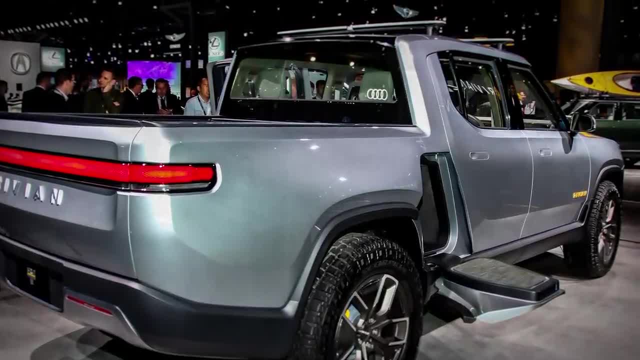 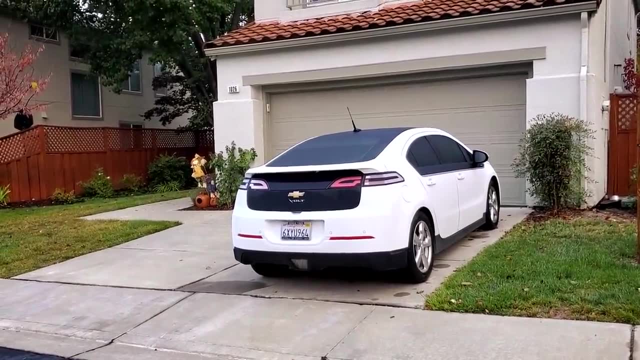 power the average American household for four and a half days. While EVs typically take in electricity, little stands in the way technologically from them giving that electricity back to the grid. So the idea is that EVs could charge at night or when renewables are performing well and 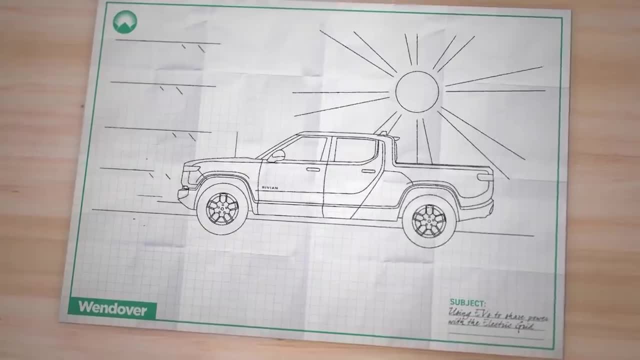 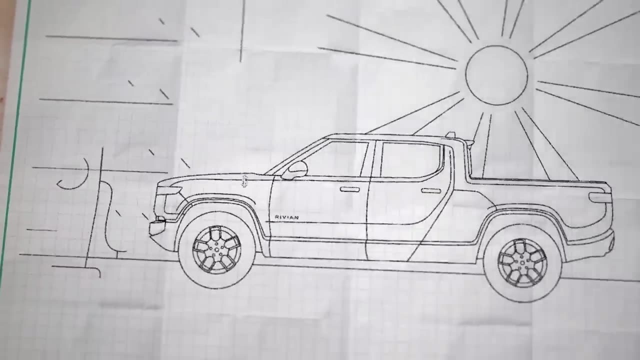 then supply some of that electricity back to the grid during the day, while parked and plugged in. In exchange, vehicle owners would be compensated a small amount by the utility company, While the real-world wide-scale economics have yet to be proven, especially in the face. 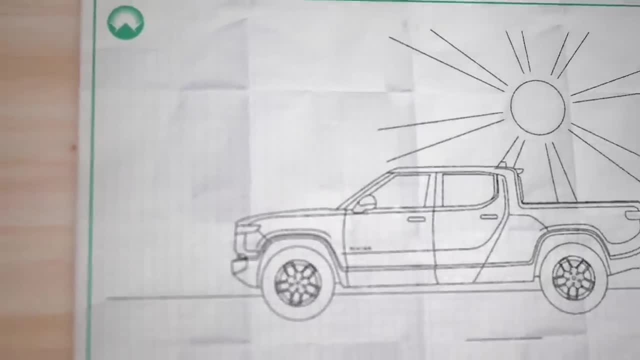 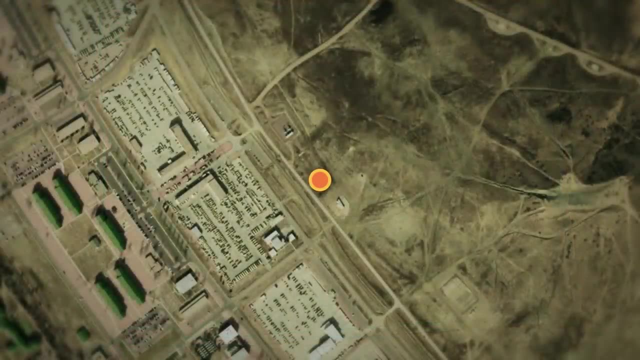 of battery degradation. this vehicle-to-grid concept could potentially play a cooperative role in the transition towards a greener grid. Now, the largest current battery electric storage system in Colorado, the Fort Carson installation, has 8.5 megawatts of capacity. 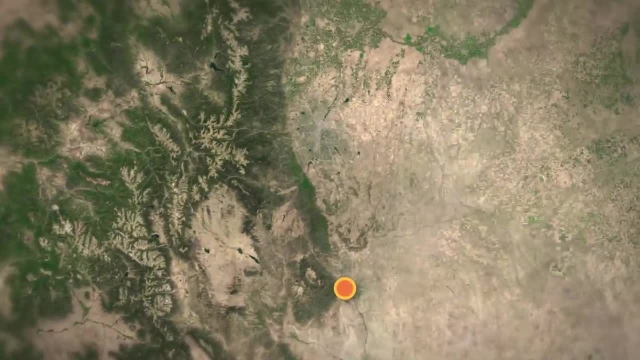 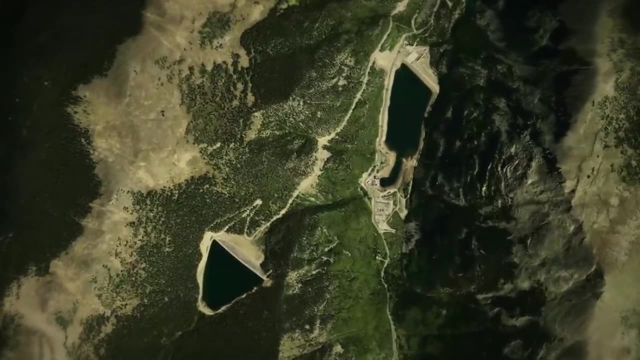 Elsewhere. it's a lot of work to do In Colorado and the state. however, there's a massive different form of battery that can power over 10,000 homes at once, And it looks like this. Water is one of the earliest forms of energy that humans harnessed, and it still represents. 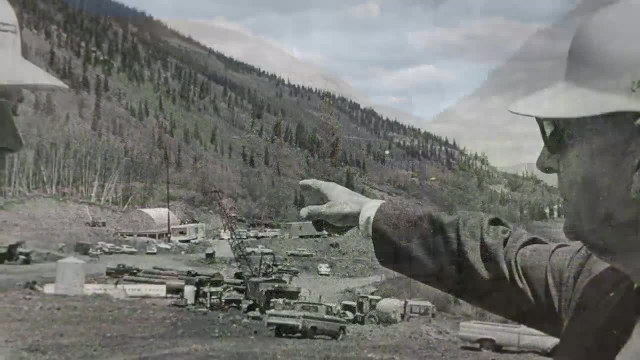 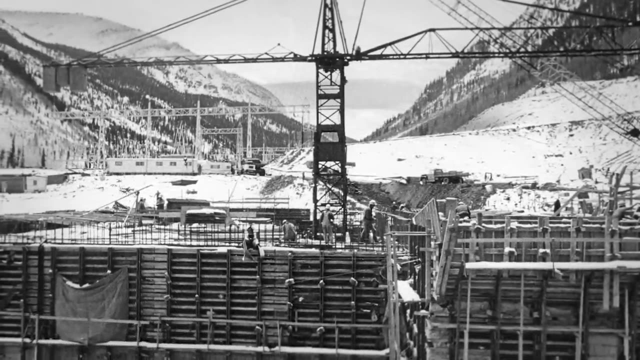 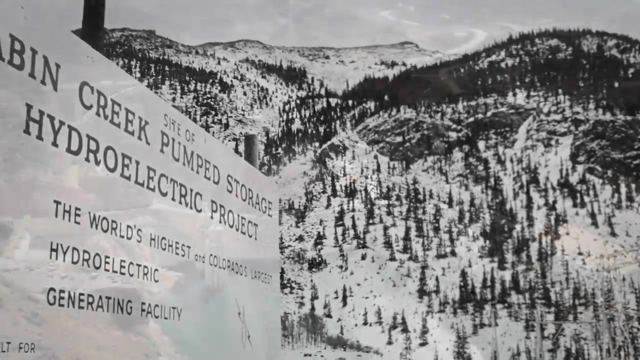 one of the best sources of electricity. Hydroelectric power is the best of both worlds. While there's certainly the potential for environmental damage from damming up rivers, the carbon impact is near zero, meaning hydro is green like wind and solar. However, it's also reliable. 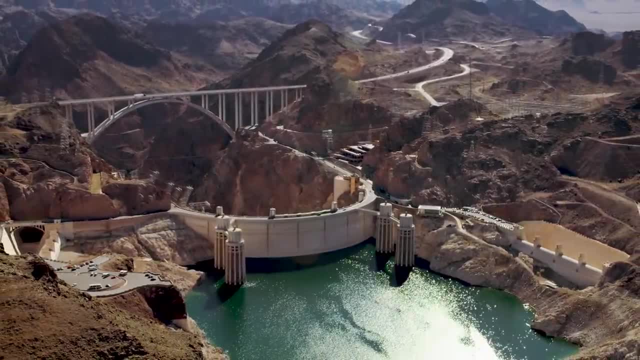 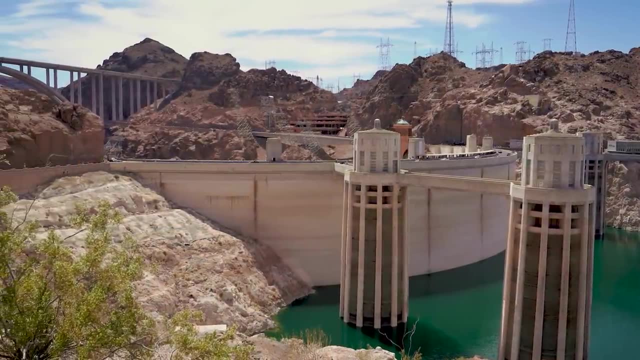 In theory, hydroelectric dams can start and stop making power in minutes, even if in practice a minimum flow is typically maintained, so they can operate like those natural gas single-cycle peaker plants, responding to demand. Of course, there's only so much water upstream, especially in a place like Colorado, which 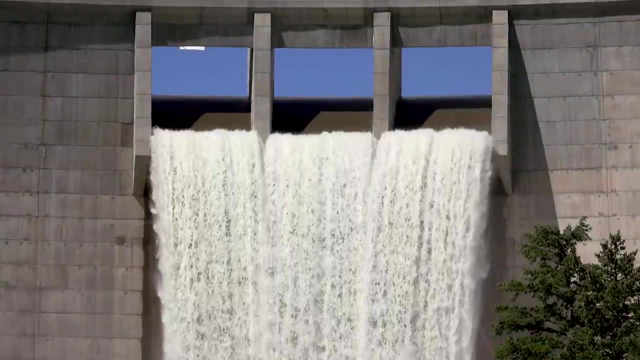 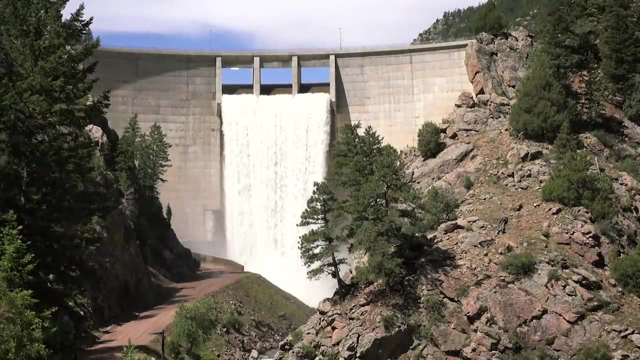 is in the midst of a 20-year-long drought, but hydroelectric dams simply convert potential energy into electric energy. There's no reason why that process can't happen. It's just not possible. That's what happens here at the Cabin Creek Generating Station. When electricity's cheap, typically at night or when wind and solar are performing at their peak, the facility uses it to pump water to its upper higher-elevation reservoir. Then, when electricity's expensive and in demand, like in the late afternoon, it will. 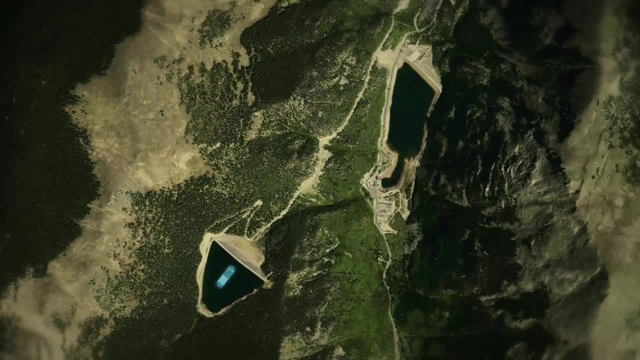 start flowing that water through its turbines out into its lower reservoir. It's essentially a form of price arbitrage, but it's one that's already helping smooth out the peaks and valleys of wind and solar water. That's what happens here at the Cabin Creek Generating Station. 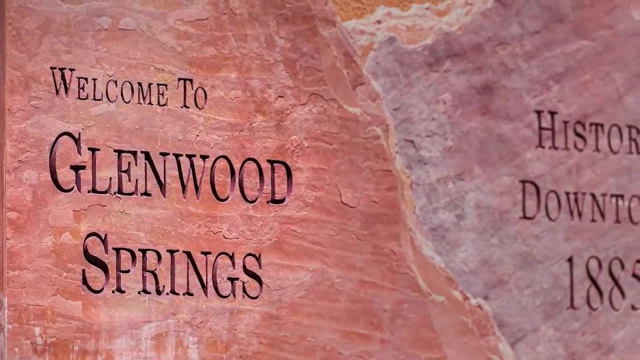 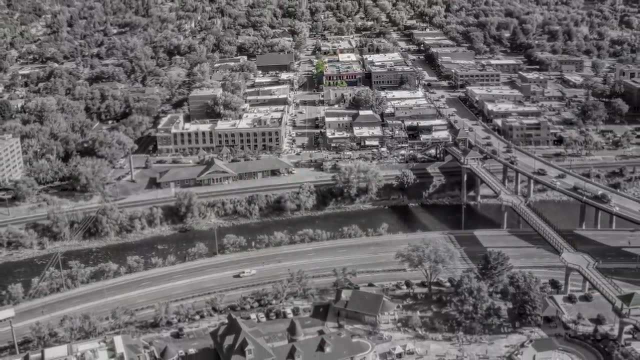 Now, no matter how well supply is matched to demand, electricity is of no use to that Glenwood Springs Colorado library until, of course, it gets there. Many have an image of power plants as something sitting just outside every town and city. 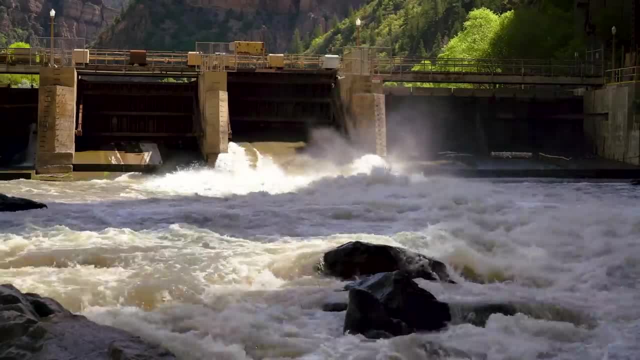 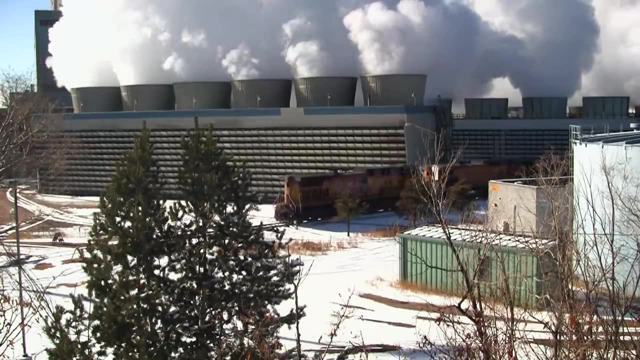 While that's how the earliest grids operated, it's hardly the case anymore. Despite dramatic declines in the past decade, some 42% of Colorado's power supply still comes from coal. That means that nearly half of the state's electricity is being used for power production. 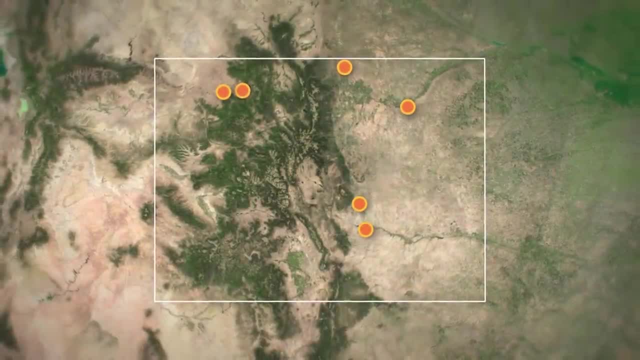 That means that nearly half of the state's electricity is being used for power production. That means that nearly half of the state's electricity is being used for power production And that electricity originates from essentially just six sites—the state's coal power stations. 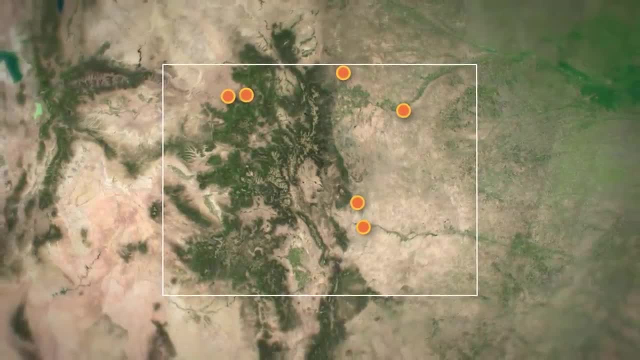 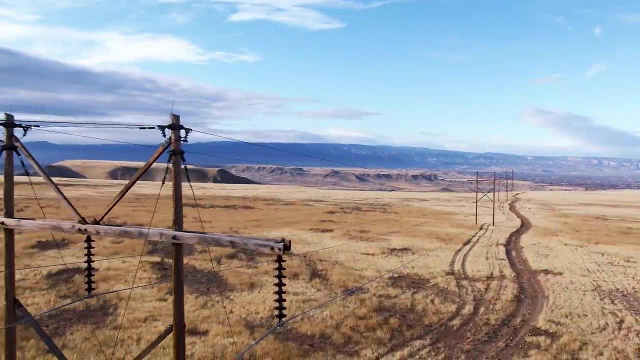 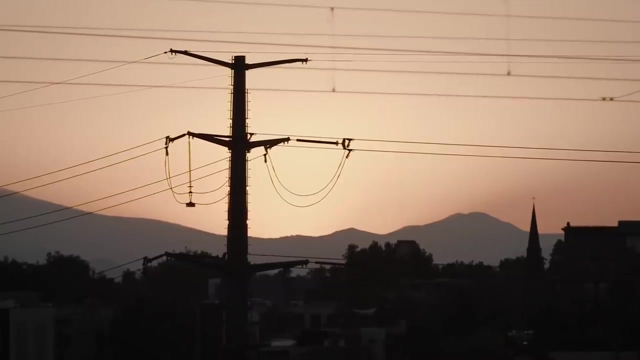 Therefore, the ability to effectively transport electricity over a long distance is essential. Now, what makes long-distance transmission tricky is simple—the further you send electricity, the more you lose along the way, typically through unavoidable conversion to heat. Meanwhile, the more centralized your electricity production, the less it costs—it's simple. 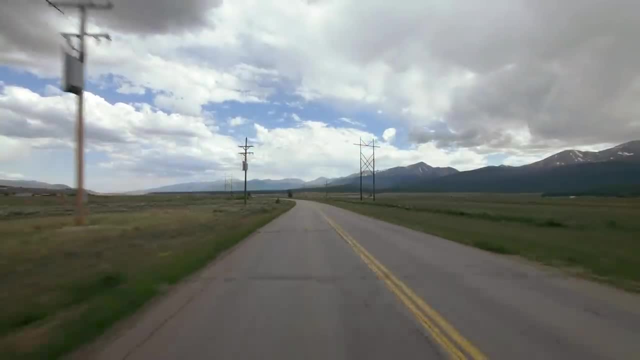 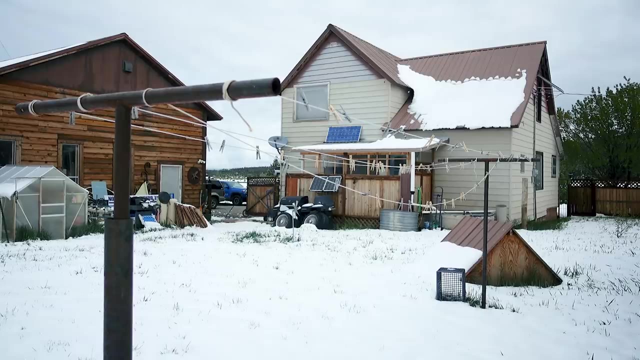 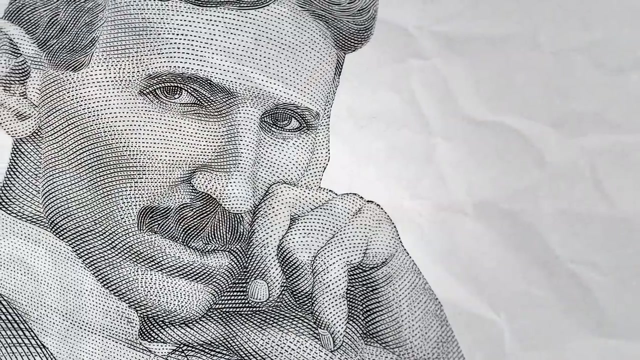 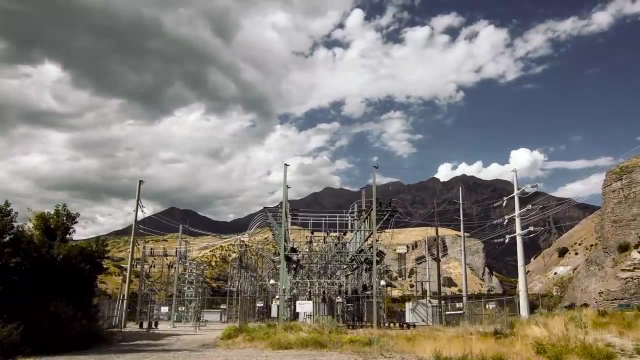 economies of scale, Therefore…. Now houses, businesses and other buildings connected to the grid all use alternating current power. A big reason why this standard beat out its direct current competitor in the days of Tesla, Westinghouse and Edison is because it's relatively easy to convert AC power between. 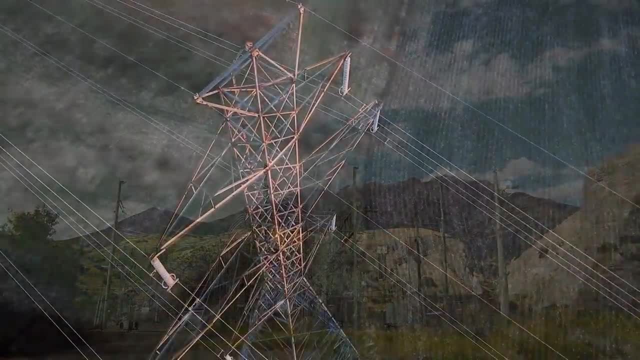 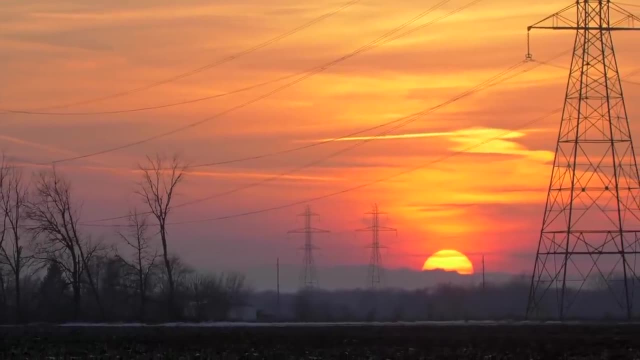 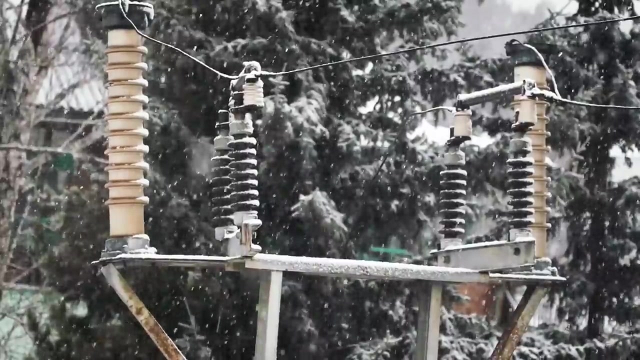 higher and lower voltages using transformers. What makes this crucial is that the higher the voltage, the less electricity lost during transmission. Specifically, a doubling in voltage quarters the power loss in transmission. That relatively simple voltage transformation allows for a more efficient electricity distribution. 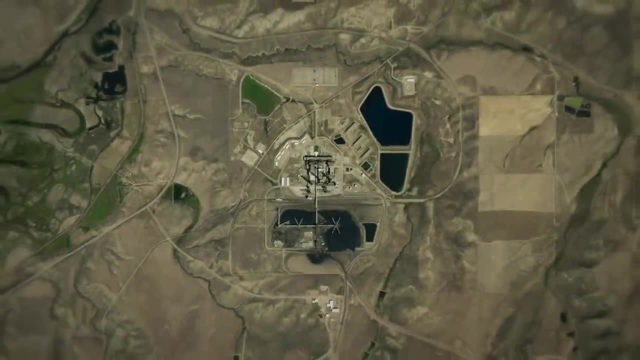 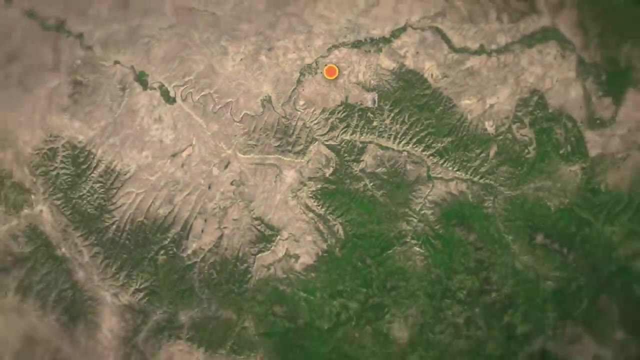 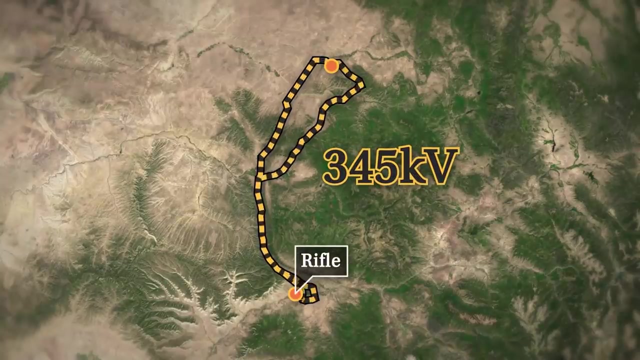 system. Colorado's second-largest power plant is this—the Craig Generating Station. It connects to some of the state's highest-voltage transmission lines, two of which head due south until the town of Rifle. Now these lines operate at 345 kilovolts, which means that, in theory, over the 75-mile 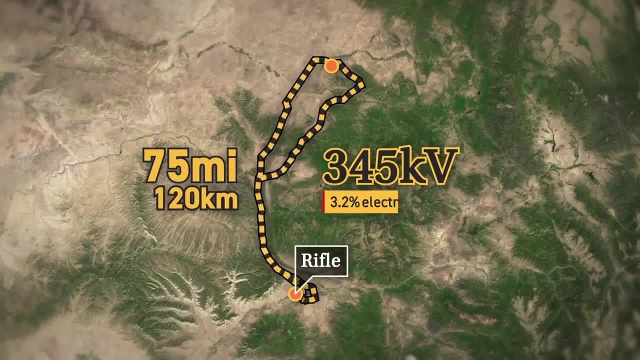 or 120-kilometer stretch from Craig to Rifle, about 3.2% of the electricity is lost—a relatively minor amount- thanks to the efficiency of high voltage transmission. However, it's the same for other lines too, So the low voltage transmission line can only connect to some of the highest voltage lines. 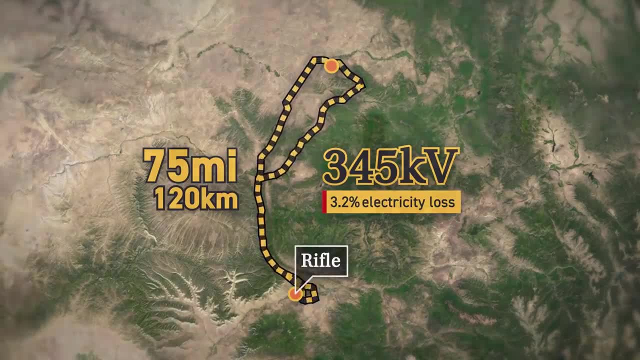 only two of these lines head due south into the town of Rifle. Now these lines operate at 345 kilovolts, which means that in theory over the 75-mile, or to the efficiency of high-voltage transmission, Other more densely populated regions which need more electric transmission capacity. have even higher voltage lines, all the way up to 765 kilovolts—the current highest voltage transmission standard in the US. Quite few of these lines exist in the US—there's one connecting Quebec to New York State, and then a larger system spanning between Illinois and Virginia. 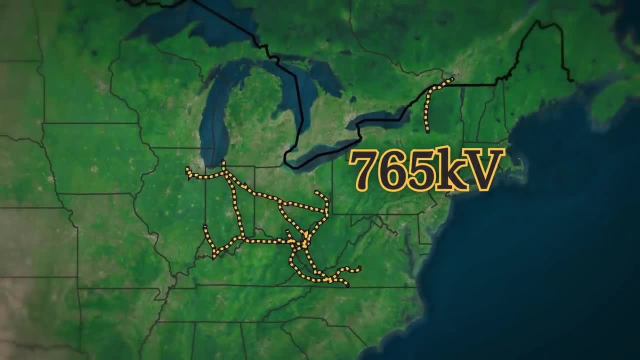 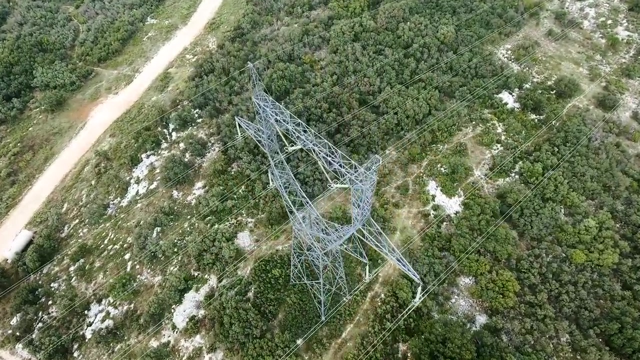 These can carry about six times as much electricity as the 345 kilovolt line between Craig and Rifle and, thanks to their high voltage, see as little as 0.6% loss per 100 miles or 160 kilometers. That means that in theory, assuming the infrastructure existed, a 765 kilovolt line could transmit. 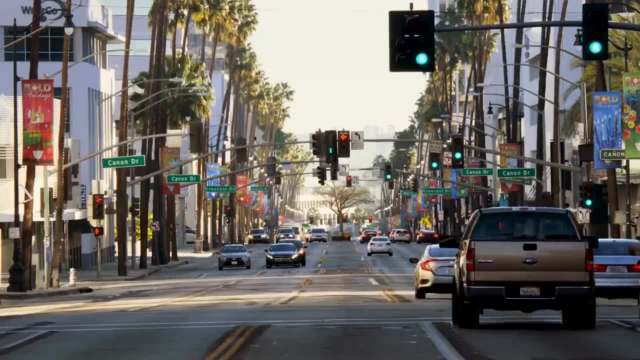 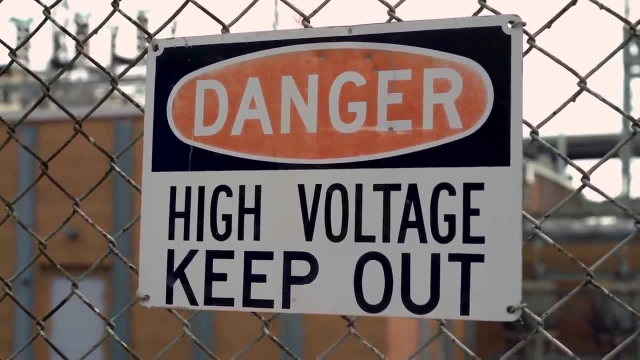 electricity from New York to LA, and about 87% of it would still be there at the other end. That's why these high-voltage lines are becoming more and more common. But what's even more efficient than transmitting an alternating current at a super-high voltage? 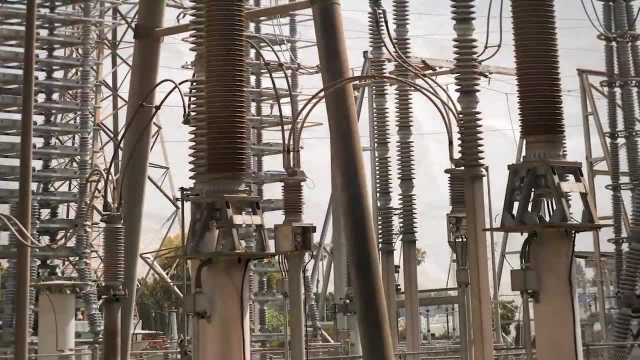 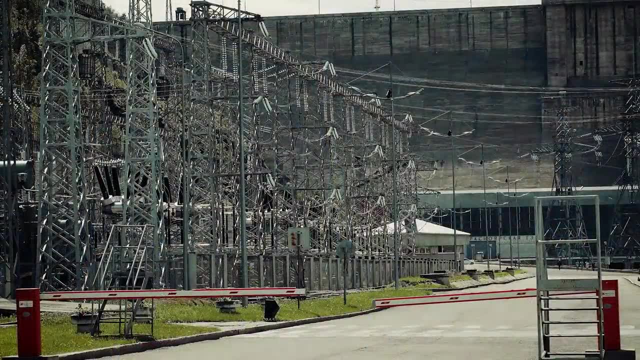 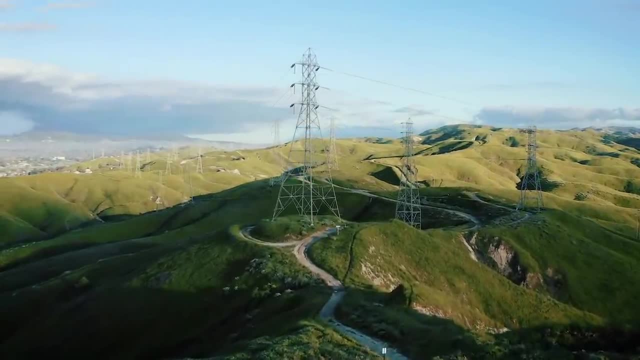 is transmitting a direct current. Of course, the difficulty with direct current is that transforming it between voltages is more expensive than with AC and for use in today's grid it has to be converted to AC power, which is also expensive. However, compared to the absolute lowest, 0.6% loss per 100 miles with the highest voltage. 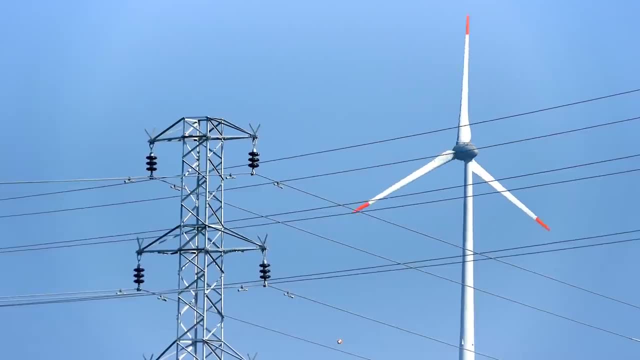 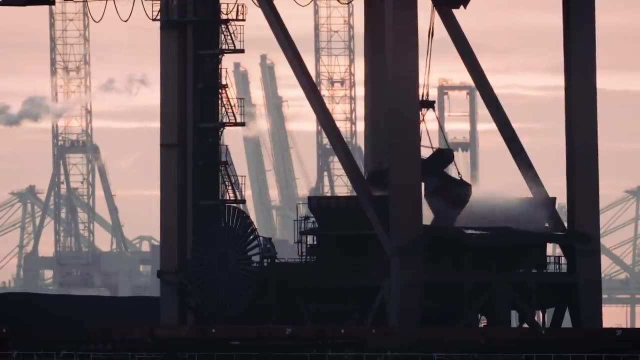 AC lines, DC lines see as little as 0.45% loss per 100 miles. Therefore, when there's a need to transmit a huge amount of electricity over a long distance, the economics can work in favor of converting power to DC at its origin and converting 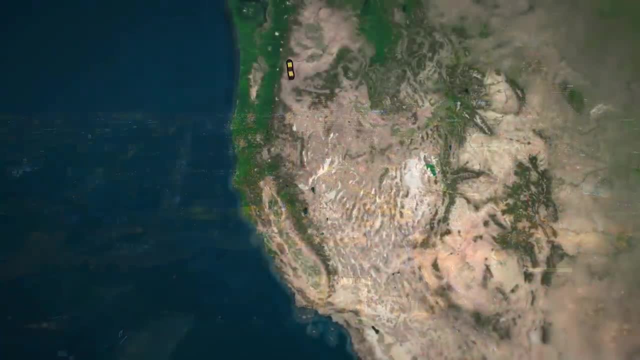 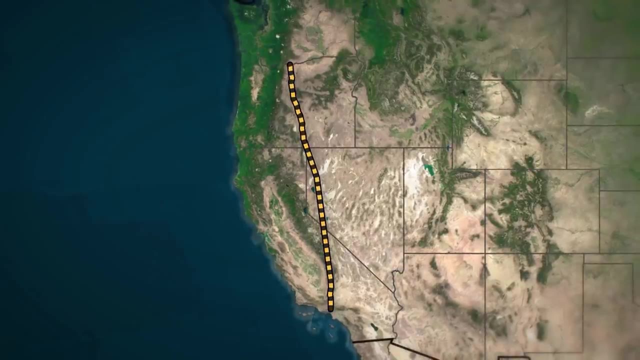 it back to AC at its destination. Perhaps the most prominent application of such a system in the US is the Pacific-DC Intertie stretching between Northern Oregon and Los Angeles, California. In the summer, the temperate northwest has relatively little power demand but generates. 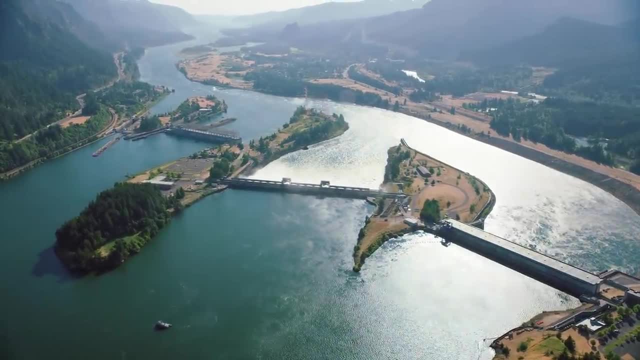 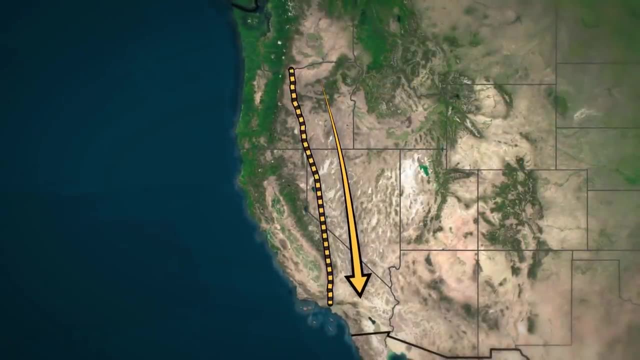 a huge amount of cheap electricity thanks to its hydroelectric dams. So the Pacific-DC Intertie sends this electricity south to power Los Angeles. That's the Pacific-DC Intertie. Meanwhile, in the winter, Los Angeles sees temperate weather and little need for climate. 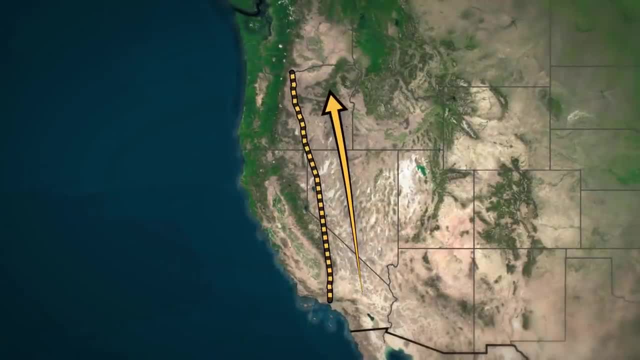 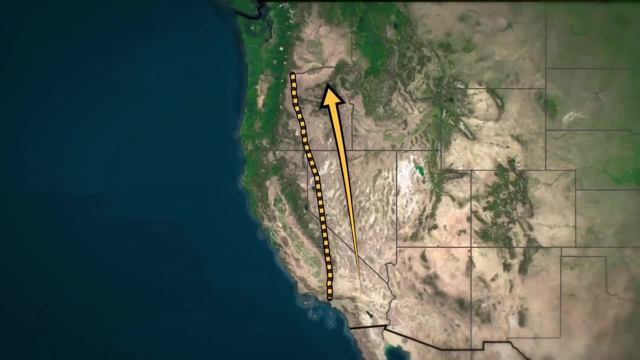 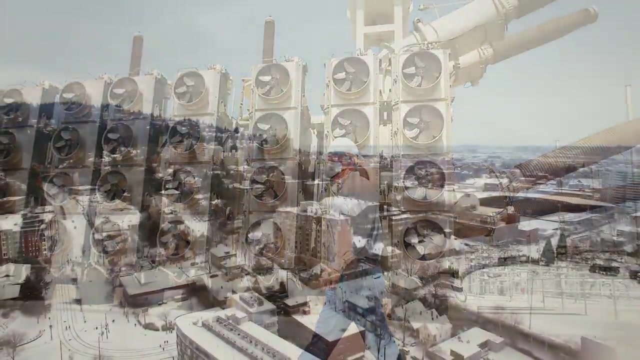 control, so it sends its excess electricity north to the Pacific Northwest to power its electric heating. Phenomena like this demonstrate why creating a greener, more efficient grid involves a proliferation of long-distance power transmission infrastructure—it's needed to balance out seasonal trends and to bring power from where it can be produced easily to where it cannot. 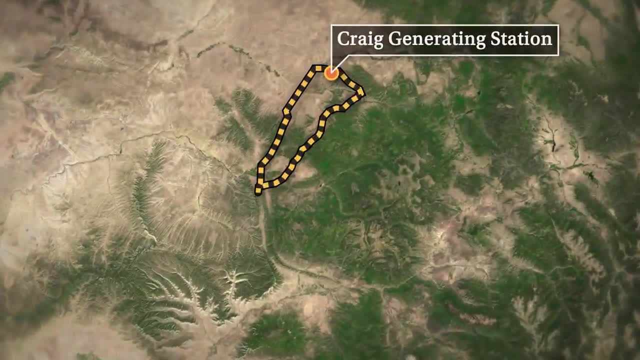 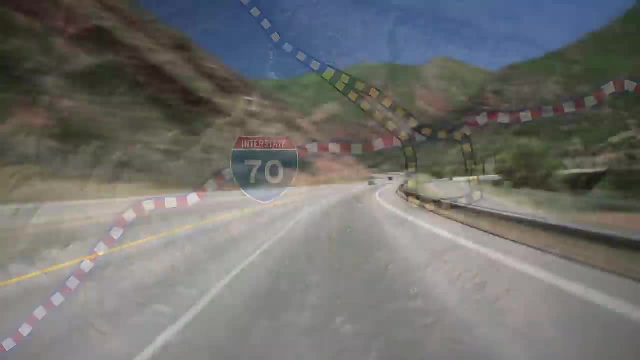 Back in Colorado, though, its relatively minor 345-kilovolt line from the Craig Power Station eventually enters this more populated area flanking Interstate 70. Here there are a number of nearby towns that need electricity, but sending 345 kilovolts. 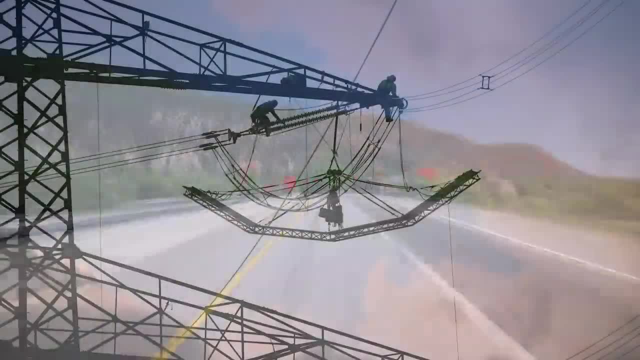 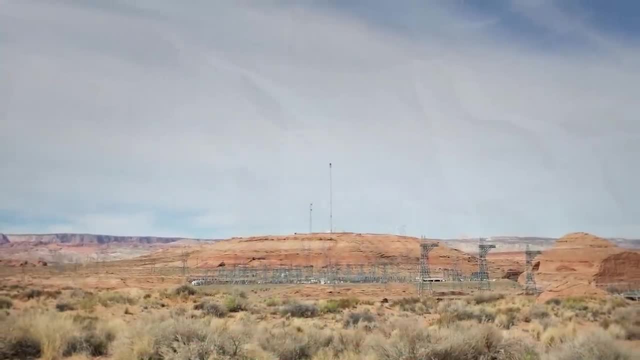 to each of these would not be efficient. That's simply because the higher the voltage, the higher the construction cost. A 345-kilovolt substation might cost $10.7 million, while 235-kilovolt-one just costs. 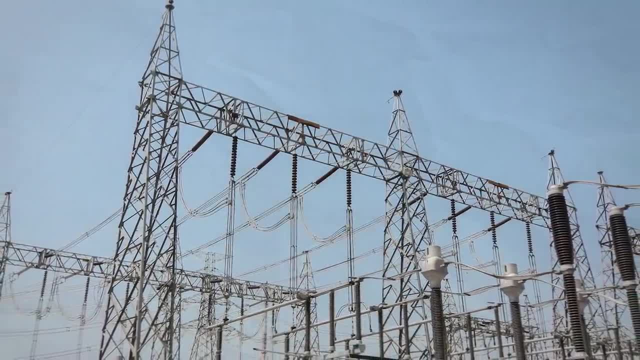 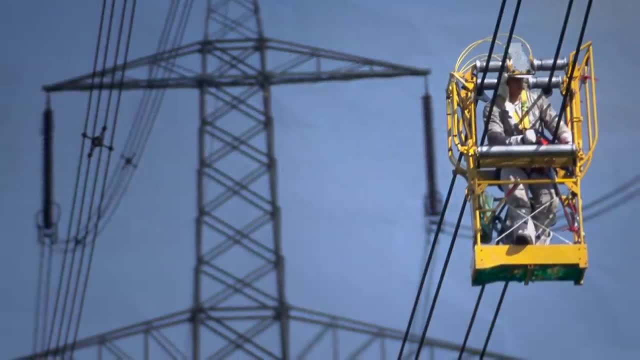 $10.7 million. Meanwhile, a 345-kilovolt line costs around $4.5 million per mile to build, while a 230-kilovolt line just $2.8 million. Therefore, even though the transmission losses will be greater, a number of substations around 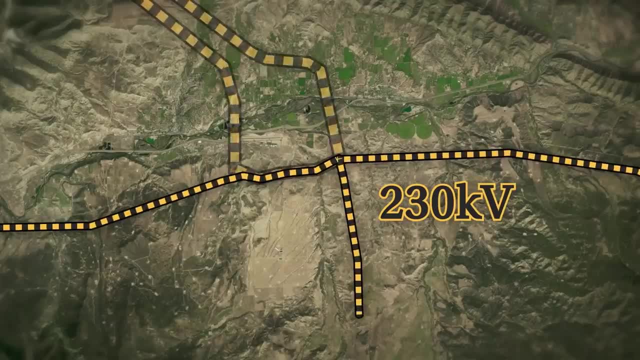 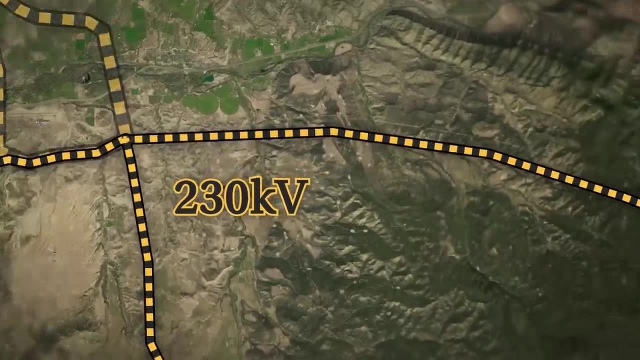 Rifle, transform the electricity to 230 kilovolts, and then smaller, cheaper lines carry the flow west, south and east, closer to its final customers, About 30 miles or 50 kilometers to the east, this line encounters another substation which 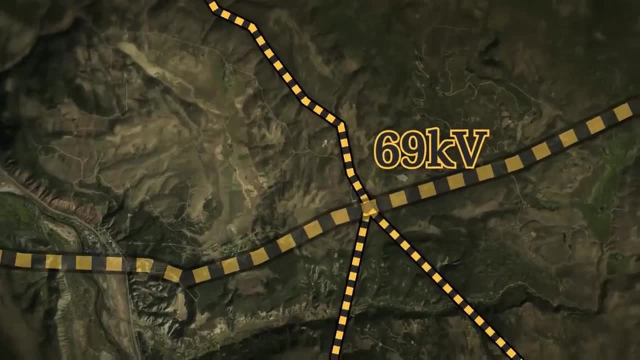 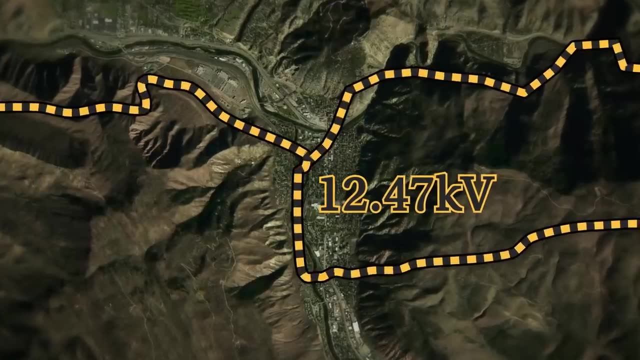 steps it down to just 69 kilovolts, and then another yet smaller line circles back towards Glenwood Springs. The power is then stepped down again to 12.47 kilovolts, before a final transformer converts it to 120,, 240, or 480 volts.